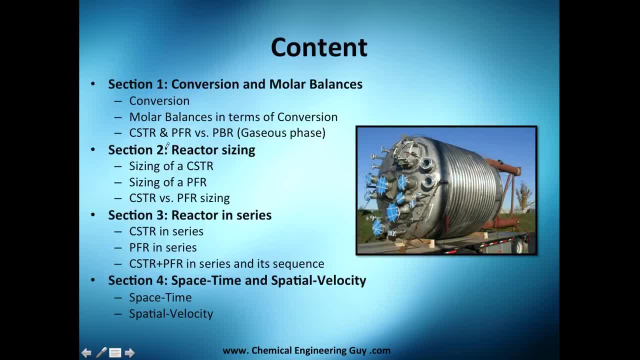 to do all this, okay, so before doing our course, I want you to let you know that this course is broken into four pieces: section number one, section number two, section number three and four. the first section is essentially just to give you a overview of conversion, some molar balances and 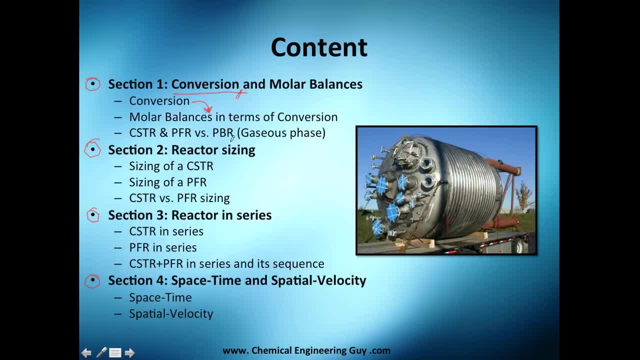 we're going to apply the conversion to those molar balances and then we're going to see some differences between the continuous-steer tank reactor, the plug flow reactor and the back bed reactor. now, that's the first thing about conversion. then we're going to see a 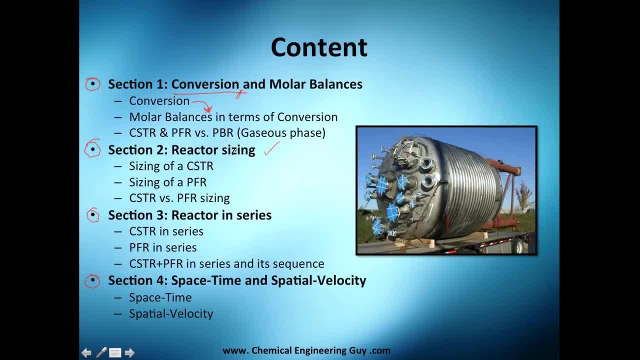 little bit of reactor sizing, especially the continuous flow reactors, which is this one here, continuous-steer tank reactor, and this one over here, the plug flow reactor. and not only that, we're going to see how they differ in sizing, how can we differentiate or see the difference between each other? advantages: 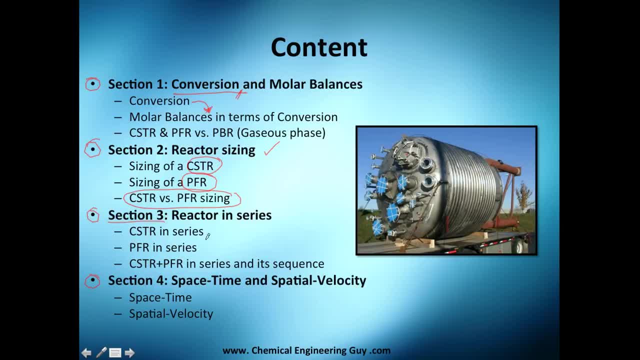 disadvantages, etc. then we continue. section number three. we're going to set up series of reactor because sometimes it's common to have different types of reactors and you generally try to get the best arrangement so you get a cheaper and low volume system. so we're going to analyze first continuous-steer tank reactors in series, then we analyze. 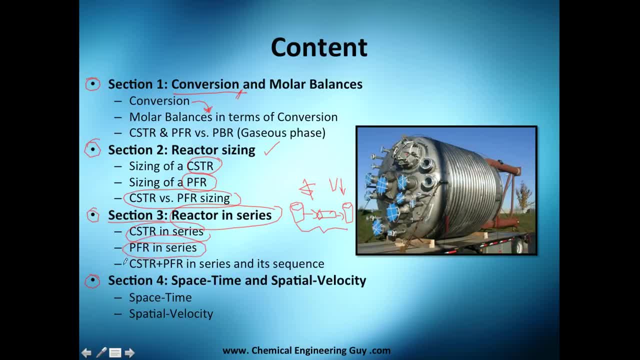 plug flow reactors in series. and then the interesting part comes here, in the continuous-steer tank reactor with the black flow reactor, mixing them, interchanging, exchanging order, everything in series and eventually you get to the best configuration of all. And finally we see a small overview of the space-time and spatial velocity which are 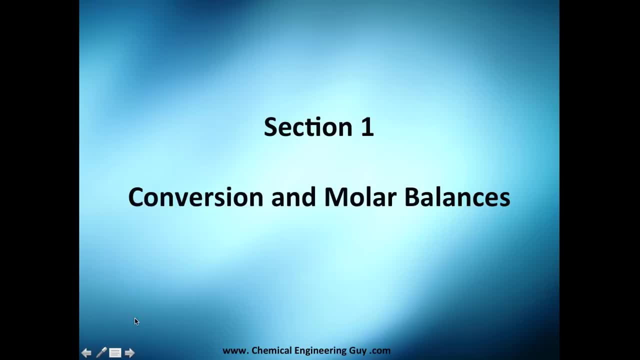 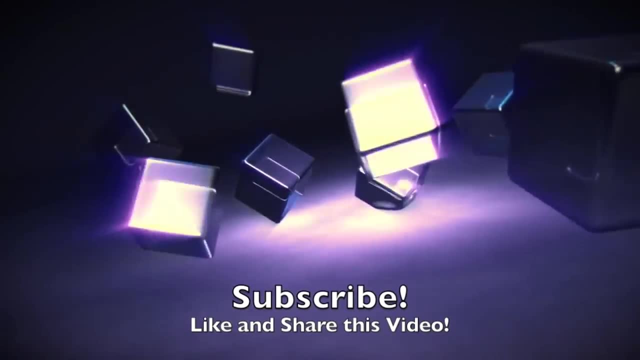 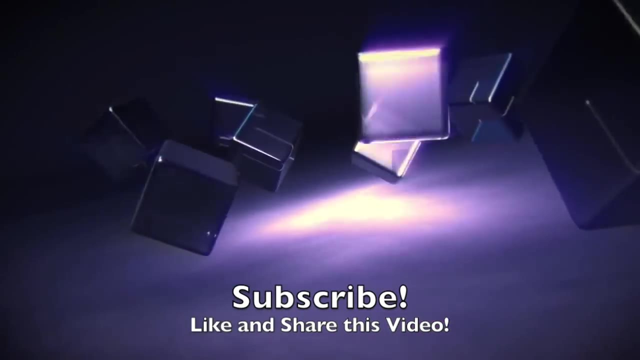 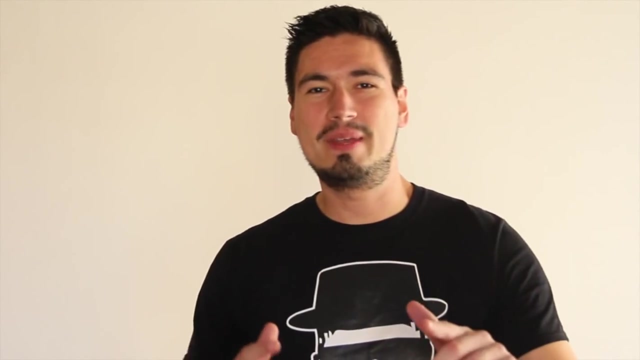 concepts easy to get and easy to calculate. So let's continue with section 1, see you in the next video. What's up, guys? it's me, Chemical Engineering Guy. so if you liked the video, why not push the like button? It really helps me to know if you're liking the videos or if I should be changing something.